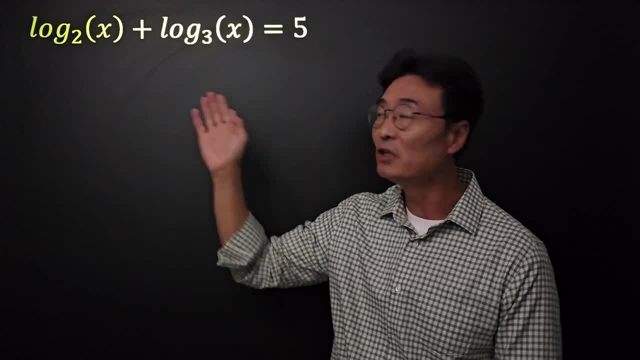 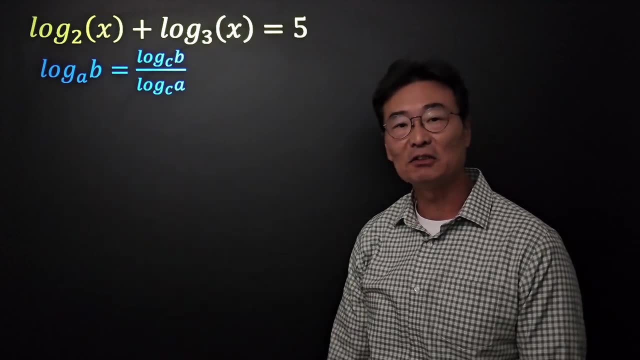 of x. It's not that hard if the bases were the same. However, when the bases are different, we have to go through some extra process. First, let's take a look at the change of base theorem which we're going to be using to solve this equation. The theorem says that if you have 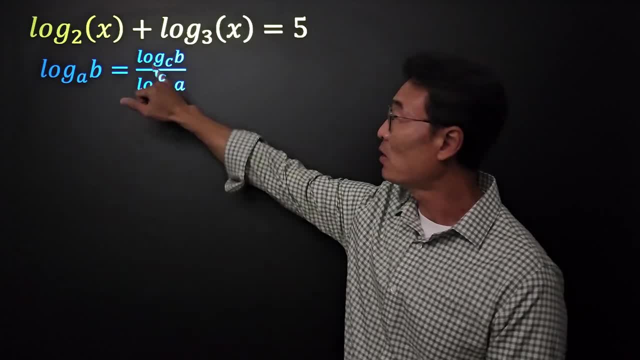 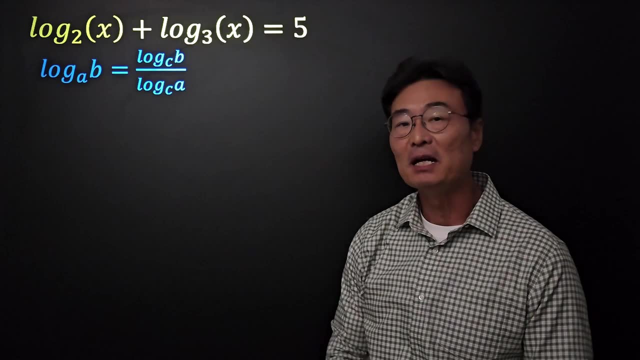 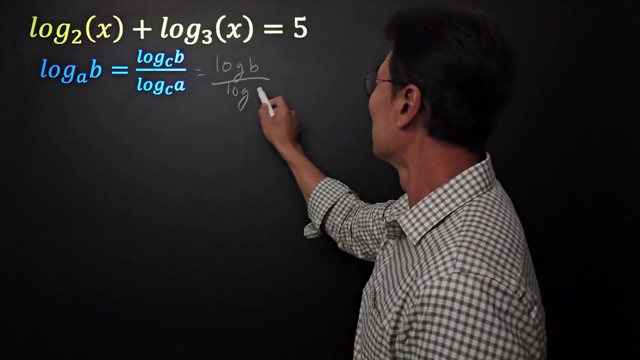 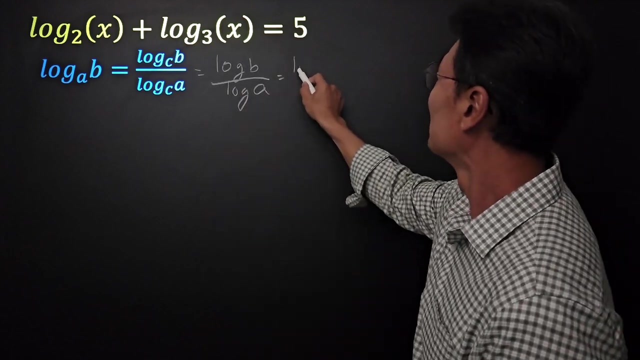 log of base a- b. it can be written as log of base c b over log of base c a. Notice, the base on the top and the bottom are the same. So the one we use more often is log of b Or the one I prefer is natural log of b over natural log of a. So when you're given log of 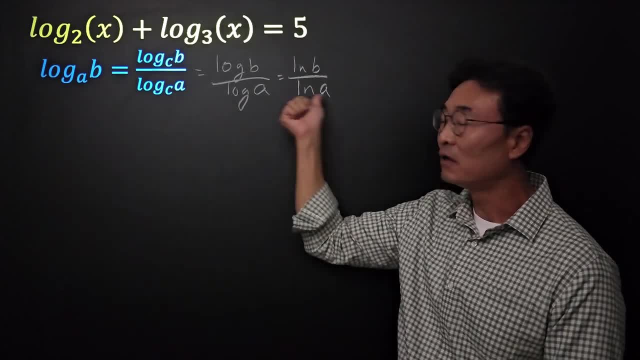 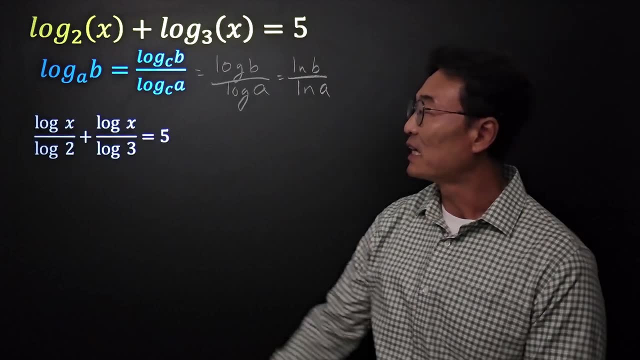 base a, b. you could rewrite it into any of these three formats. Then let's take a look at that log of base 2x. We could change that as log of x over log of 2.. Once again, notice, I'm using the ones. 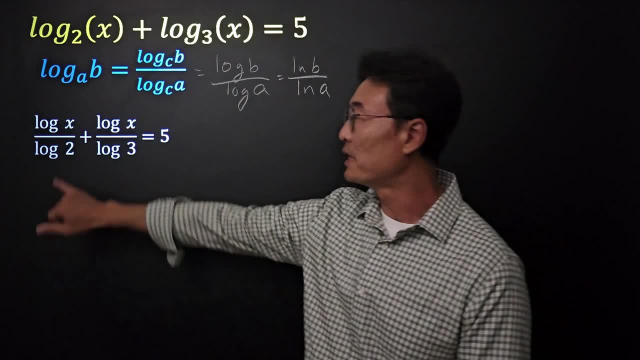 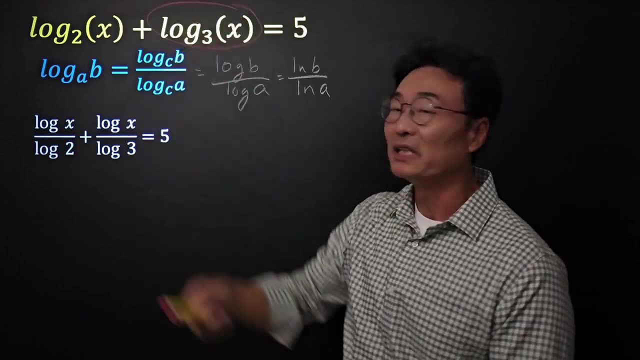 with the base of 10 on the top and the bottom. What's important is that we don't have to write the arguments that the base on the top and the bottom or the numerator and denominator are the same. Also, when we see that log of 3x, I changed it into log of x. Notice the 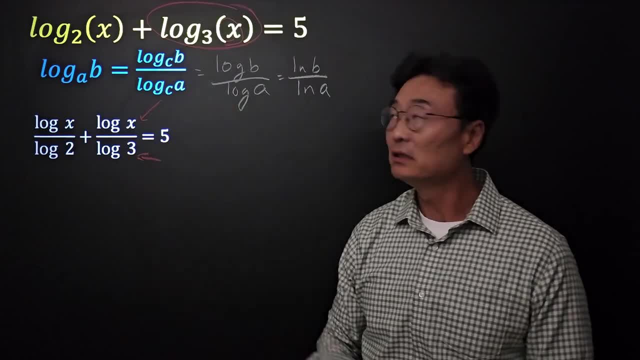 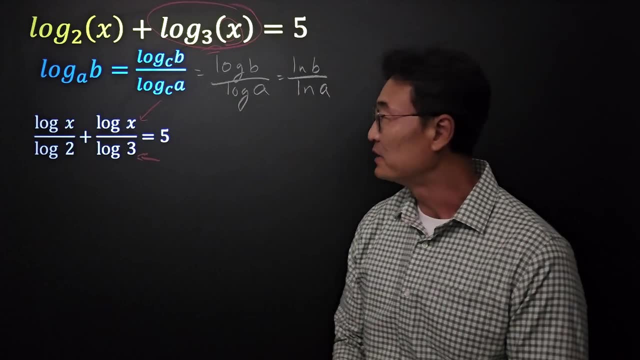 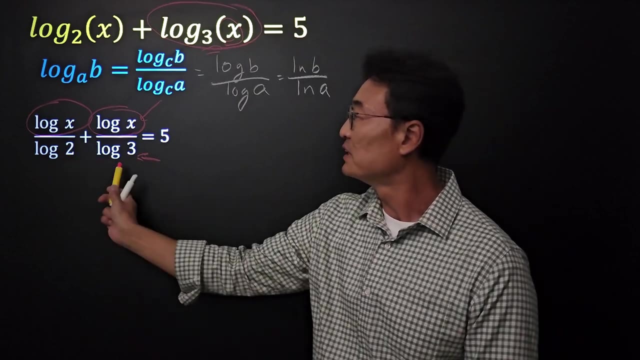 argument goes on the top- Log of 3,- or the base goes on the bottom And, of course, equals 5.. Next, notice that we have the log of x here and log of x here. So what we want to do is we want to factor out the log of x from these two fractions. 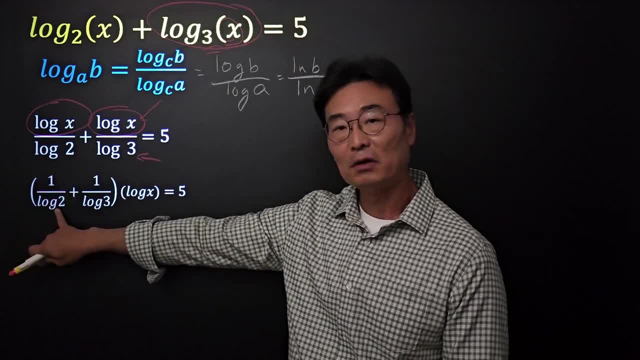 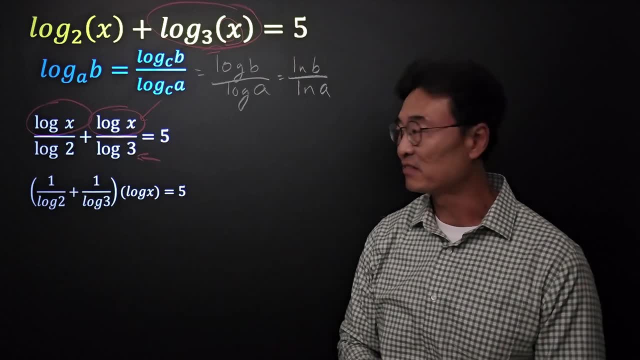 Making it into this, where we have 1 over log of 2, once we factor the log of x out, And also we have 1 over log 3, once we factor the log of x out times. log of x, of course, equals 5.. 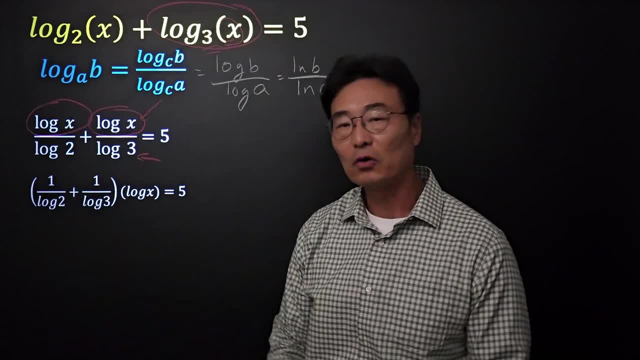 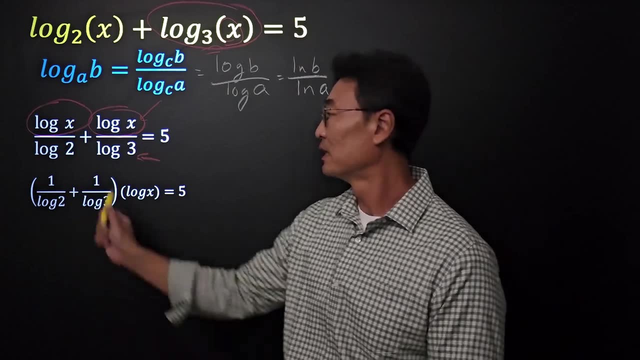 Then at this point, we don't want to continue to have this 1 over log 2 plus 1 over log 3 with us, because it's just too much work. We want to plug this, Everything that you see in this parentheses. 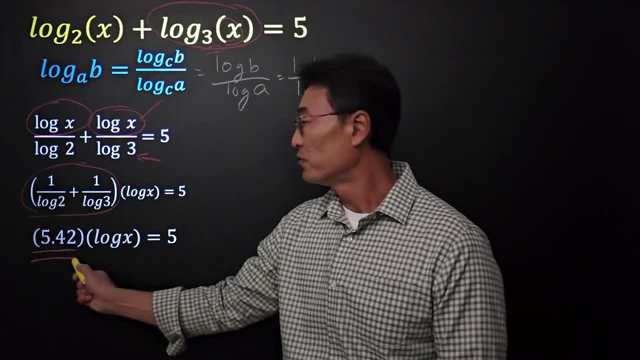 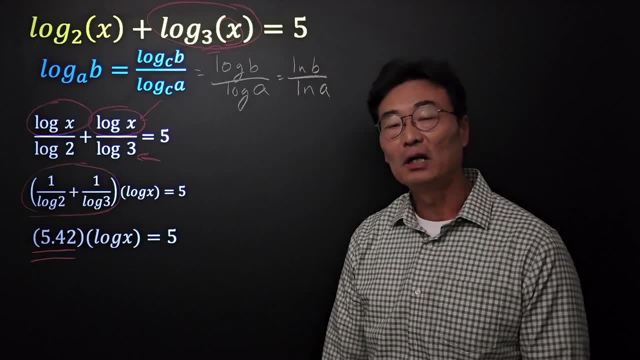 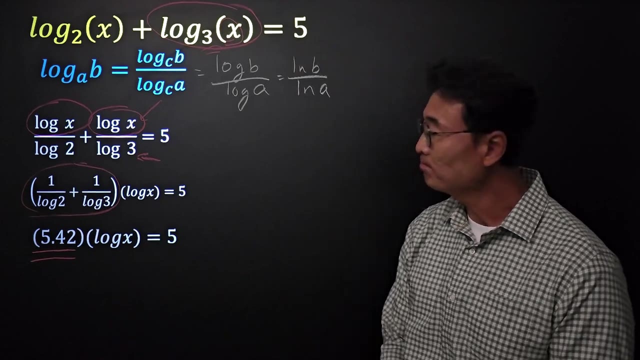 in the calculator, where we get 5.42 if we round it up to two decimal places For a more accurate answer. you can round it up to three or four decimal places as well, But usually two decimal places will do the job.